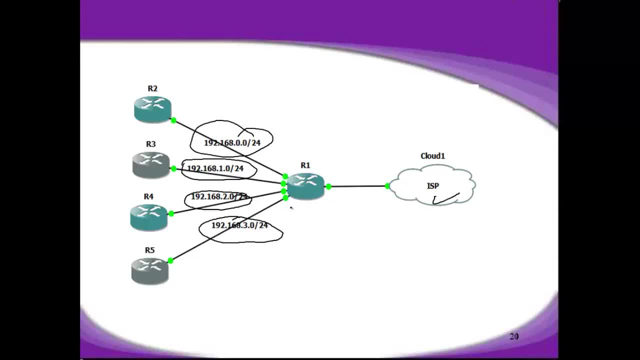 This is my corporate network out here. So now the question is if I am going to advertise all those entries by the router, all those entries by the routeror the specific origin summarized entry. so super netting is actually going to take these all four. 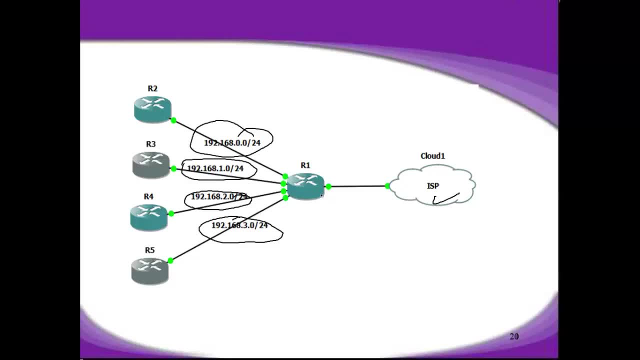 networks and going to summarize it into one network entry. this is how you are reducing the number of total network entries which are to be advertised by this router to the corporate network. so how to do that? so first of all, let me write down all four networks which I had there in the scenario, and these four 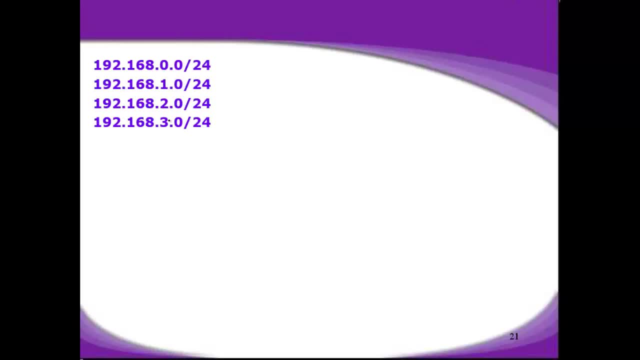 networks are 192.168.0.0. 1.0 and 2.0- 3.0 with slash 24 values. this slash 24 is nothing but the networking bits, that means ones. so that is basically a Subnet mask for these network entries. so the steps which are required to do. 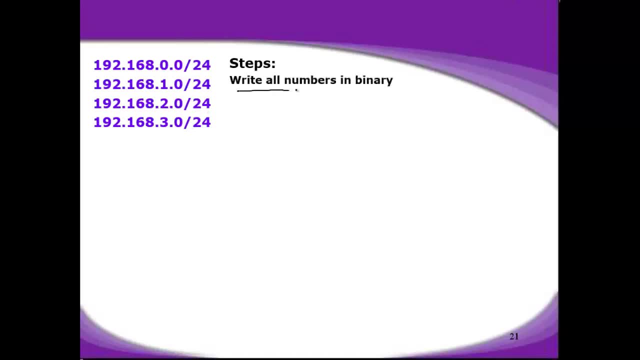 super netting. the first step is write- write all the numbers in binary. so I need to write all these numbers into the binary. so this is these binary. so this is the burnera number which I have given tickets. so I am going to write all the number in binary. so this is the burnera number which I have given. 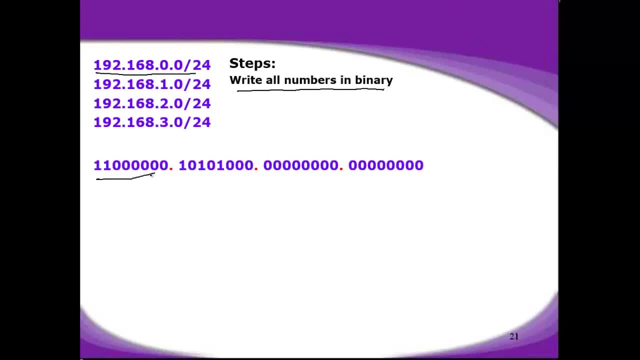 binary for this number. So how to write that? we already have discussed that. So we have the table: 128,, 64,, 32,, 16,, 8,, 4, 2, 1.. So in order to write down the binary for 192, I need to add up these numbers so that I could get 192. 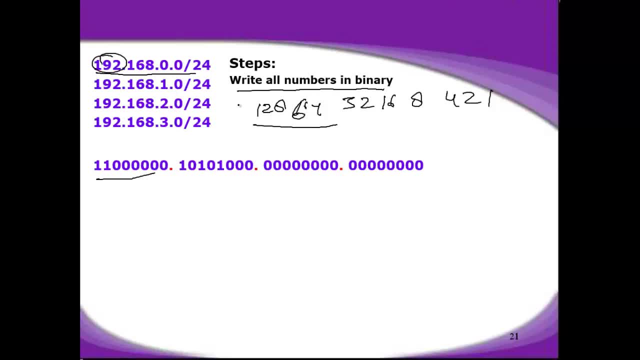 So 128 plus 64, these two are making 192.. That means I need to put 1 here and remaining I need to put zeros. So this is how I got this number, this binary number. So I need to write the binary for all four numbers. So this is the first step. So I have written down all the binaries for all the numbers. 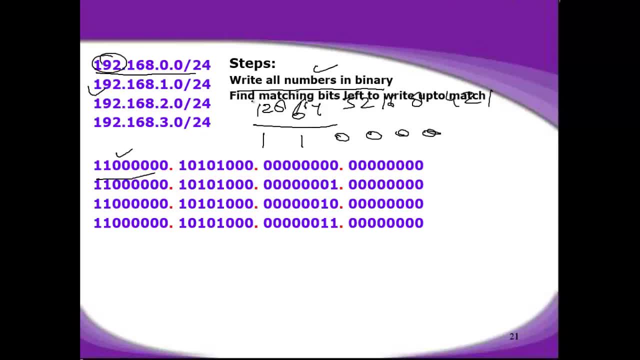 Now the next step is find matching bits left to right Up to a match, until you don't find the different number. So this step is you have to start matching the bits from left to right up to the match, as long as it is matching. So if you look here and you compare these four numbers, you can see here that these are the bits which are matching out of these numbers. 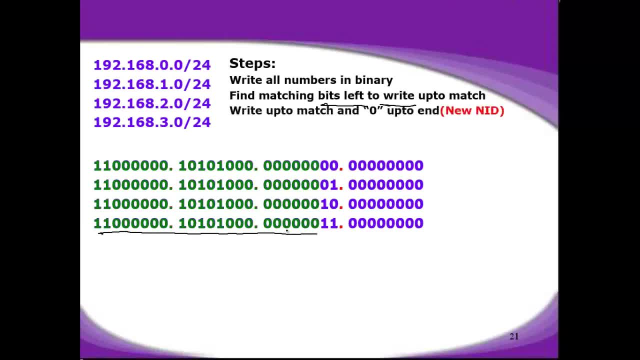 So, after matching it, you have to go to the next step, and the next step is to write up the match the same number, Whatever the number is there. write that number down plus put 0 up to the end. So the number which I am going to write this way is going to match to the original number. 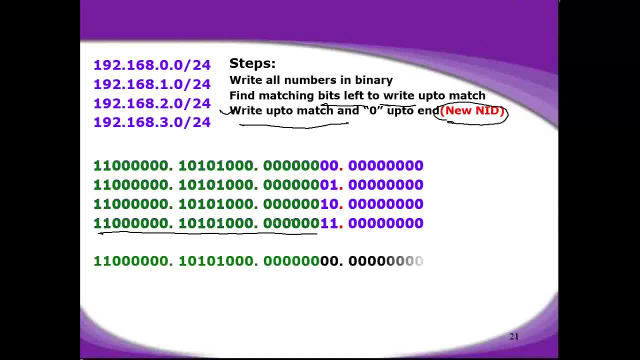 be my new network ID. so you can see here in this number this is the matching part and from there because it is different from here. so I am changing and I am putting all those zeros there, just zeros as per this step, and if you write down the decimal equivalent to this number, that is going to be 192 for this and 168. 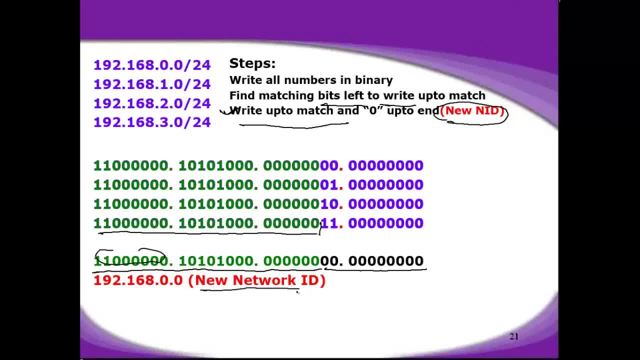 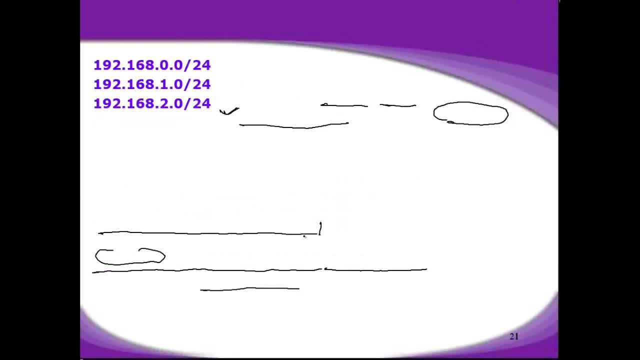 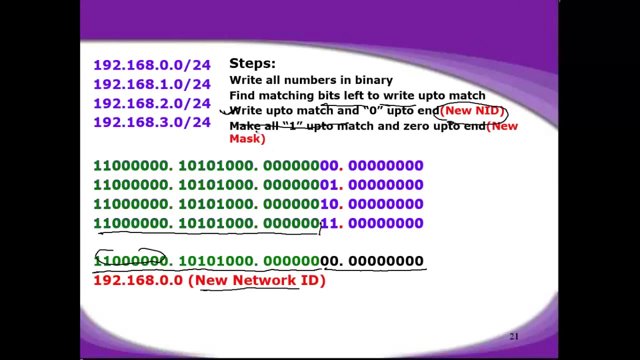 0 and 0. so this is actually the new network ID which I am going to advertise from my topology, which I told you the scenario. so I am going to advertise that network ID which we have calculated from this calculation by using these three steps. now, next step and the final step is that you have to make all once up to 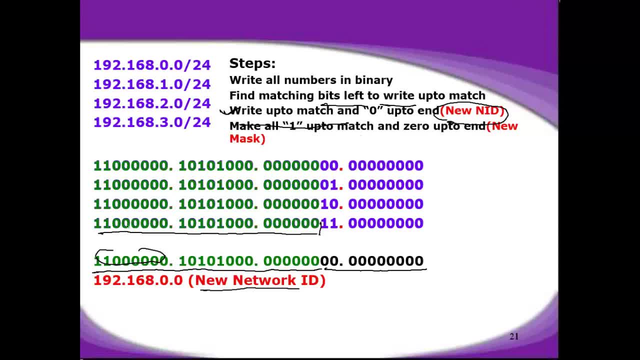 the match on all ones up to the match, and then you have to put 0 up to the end. so by doing this you will be- you are going to have the new subnet mask. so if you do so, then the matching bits are up to here. that means you are going to put all ones as per the 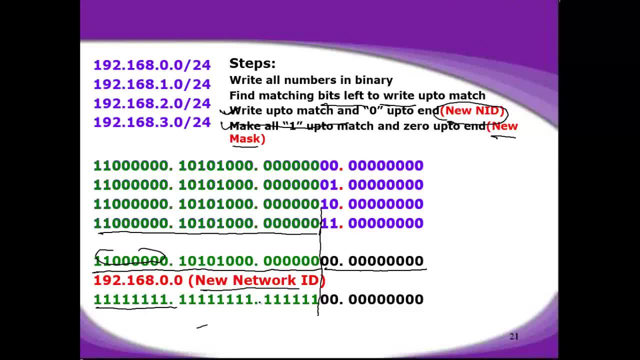 step. so that is going to give you 8 ones, 8 ones and 6 ones, that is, 22 ones and the remaining zeros completing 32-bit address. so if you write this in decimal, that is 255, 255 and 252 dot 0 and this is new mask going to be used with this. 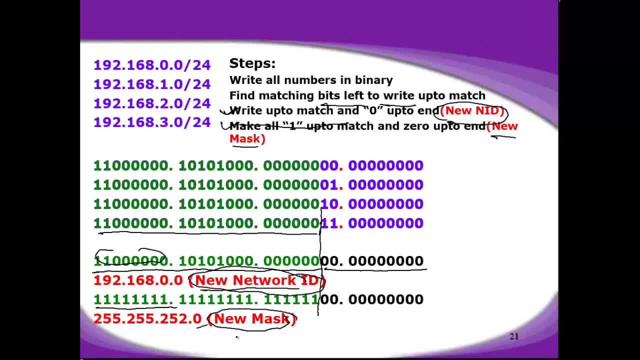 new network ID. now, one thing to note here is that in order to get this subnet mask, you are actually having this number 6 ones and 2 numbers, two zeros. so if you calculate the decimal equivalent, that is going to be 252. from the same formula: 128 plus 64 plus 32, plus 16 plus 8 and plus 4. now this is the last value I added. 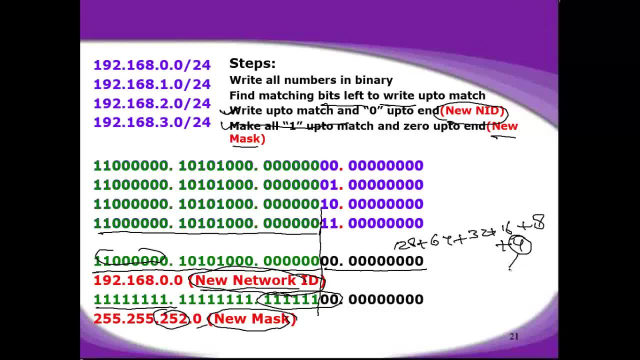 in order to get this number and this value is important to me. this value is the block size. by using this number, I am going to have next network with this mask, so we will see that in a moment. so this is the network entry, or the summarized entry, or the super net entry with: 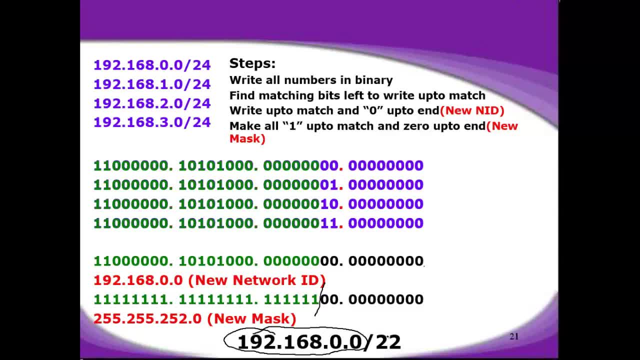 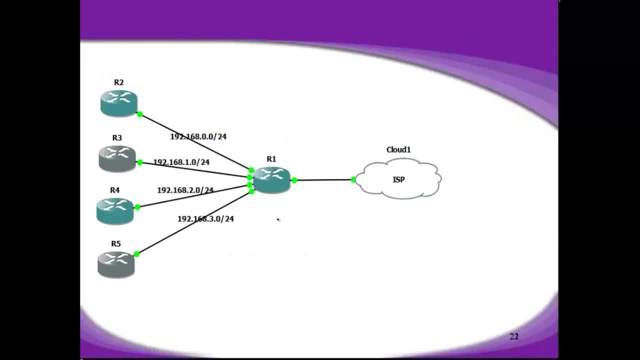 slash value of 22. that means this is the mask, new mask. so this is the entry you are going to advertise you for networks, but now you just have one entry to advertise to the corporate network. and the second and big, different, big benefit is that it is used to minimize the size of the routing table. of course, 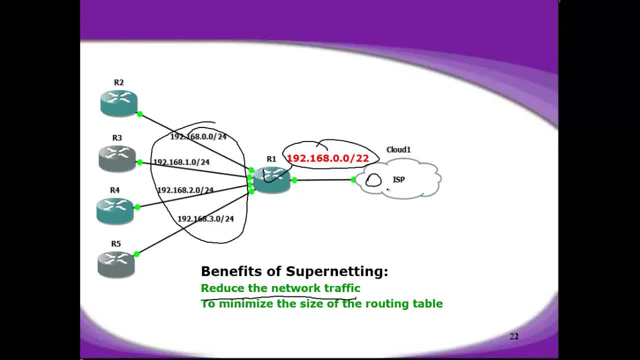 the routing routers here in the corporate network. they are going to have more burden if, if you don't minimize these all entities, because you you may be having hundreds of networks out here and instead of advertising all those hundreds of networks you are just going to advertise few entries, depending.